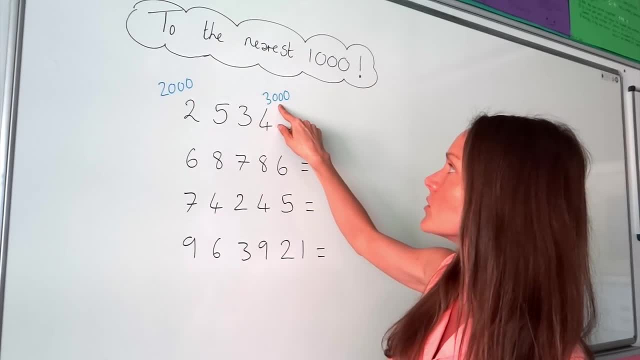 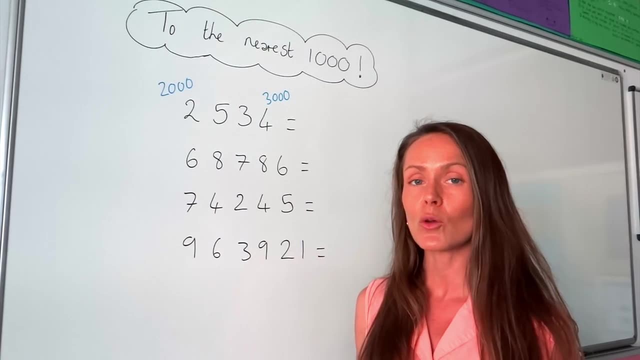 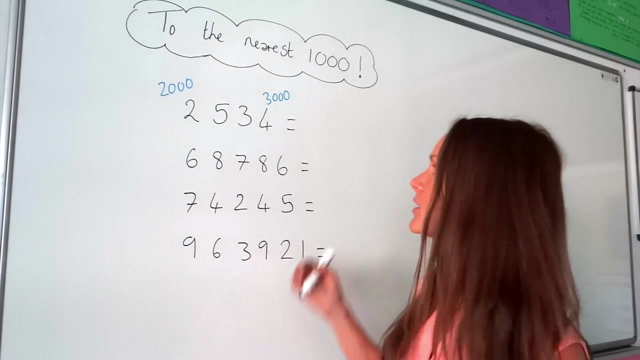 number falls in between 2000 and 3000.. So our job is to round this number up or down to one of these, and we have to round it to the one that it's closest to. So you might already be able to see which one it's closest to, which in that case is great, and you can just write down the answer. 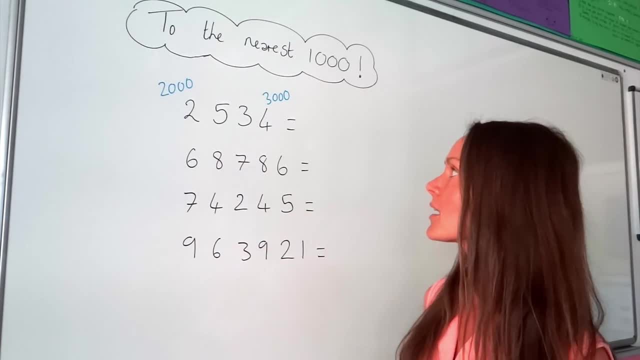 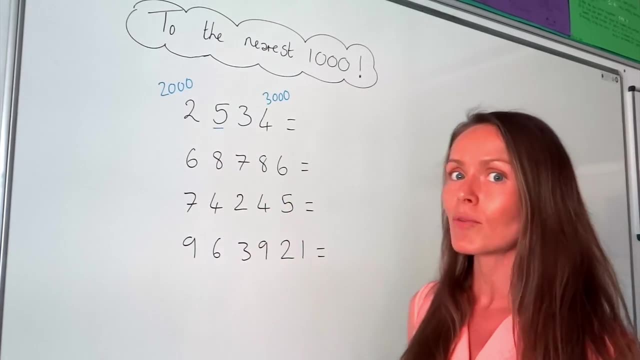 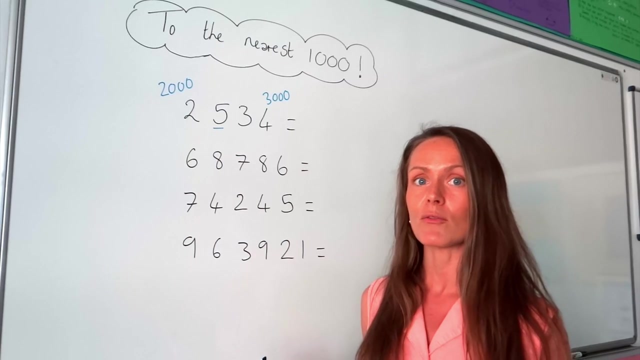 but if you're not sure, what you need to do is check the third from the end number. So this one here, so third from last, and remember when you're rounding, if you see the number five or a number that's bigger than five, then you need to round up, and if you see a number that's smaller than five, 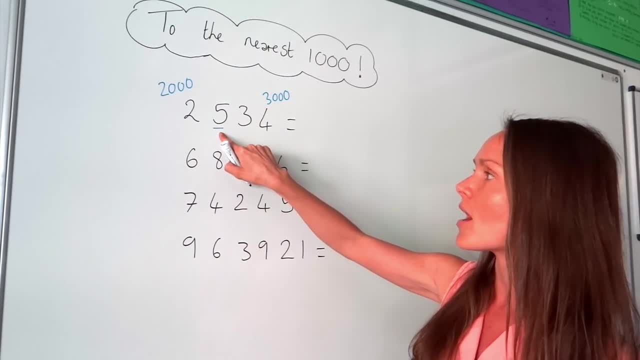 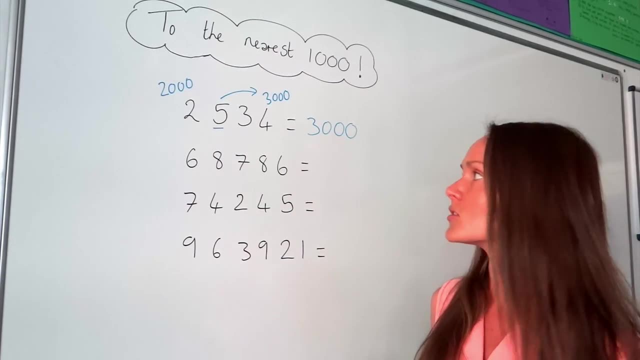 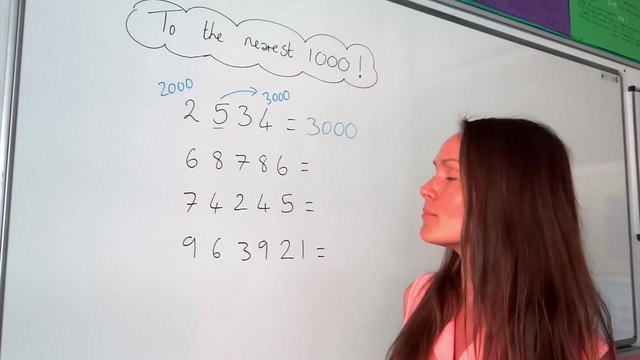 then you don't round up So in this one, because we have the number five. that means we round up So in the first one. the nearest thousand is three thousand, but maybe you already spotted that at the beginning, which is great. So on to the next one. I'm going to use exactly the same method and I'm going to write: 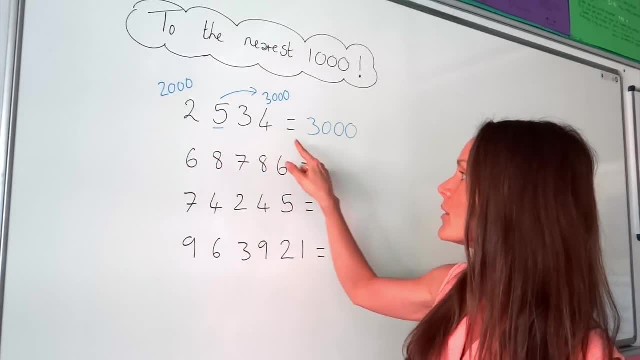 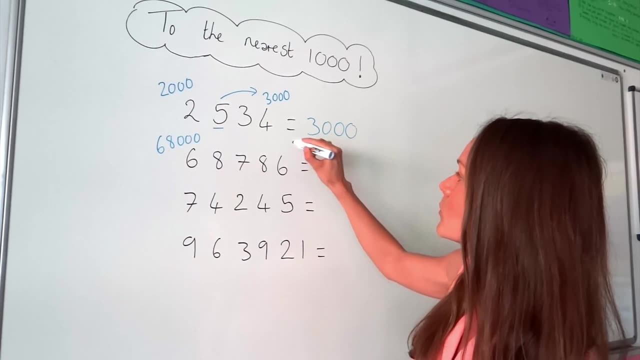 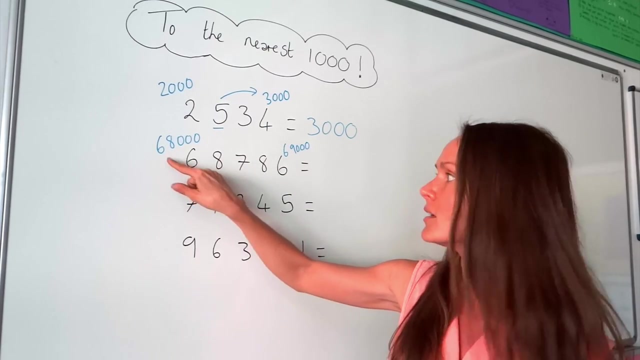 down the multiples of 1000 that fall either side of this number. So the smaller one will be 68,000 and the bigger one will be 69,000.. So if you're not sure how to spot those multiples, the smaller one is just the number that's closest to 1000.. So if you're not sure how to spot those multiples, 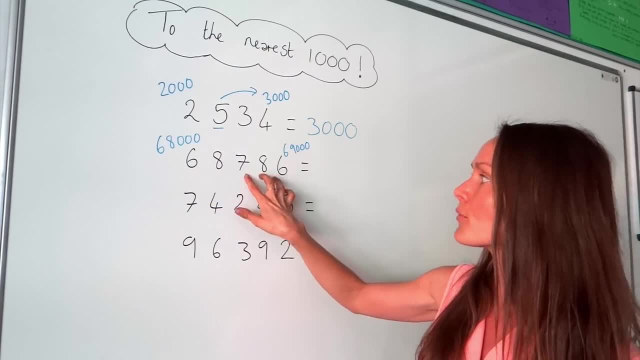 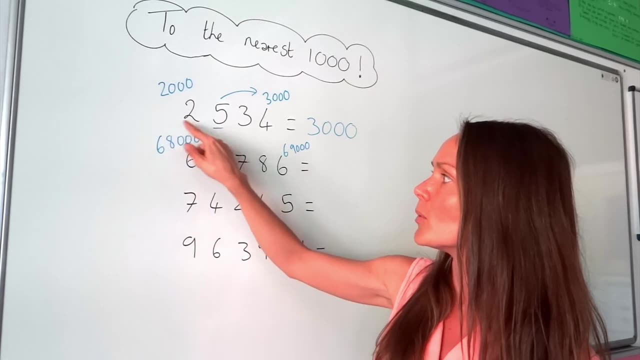 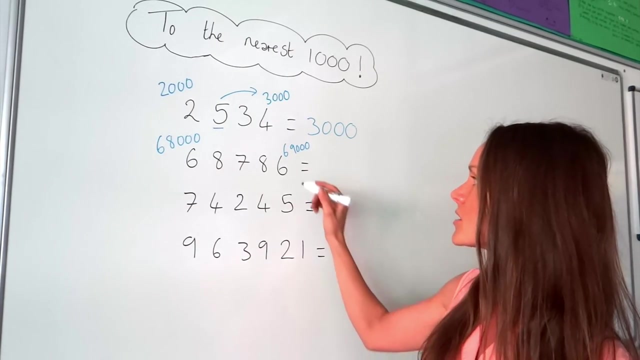 just this number here written out, but the last three zeros or three numbers turn to zeros, and this one over here is just the left hand number there, but plus a thousand. So just like before you're going to check the third from last number, so one, two, three, so that one and again because this 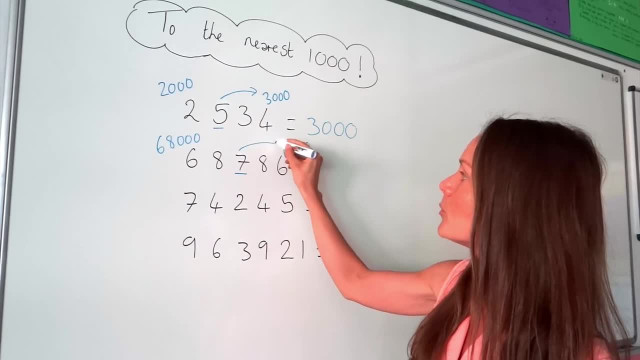 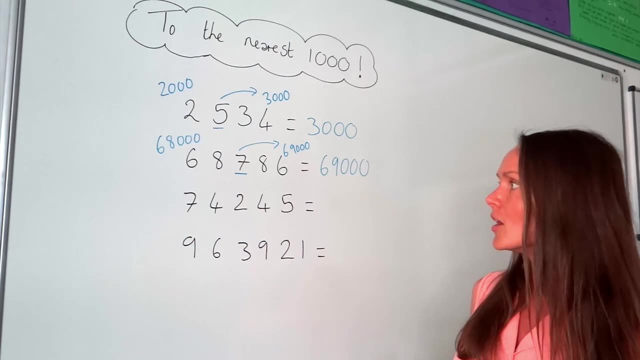 number is bigger than five. that means we're going to round up in this question as well. So the nearest 1000 is 60.. Alright, on to the next one. I'm going to use the same method. I'm going to write down the two. 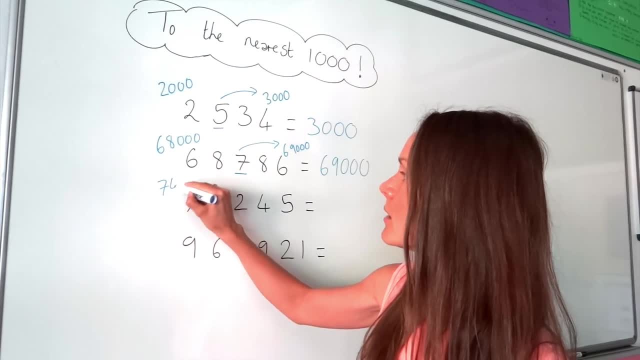 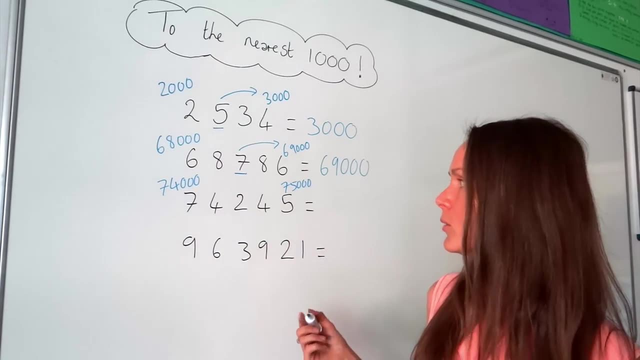 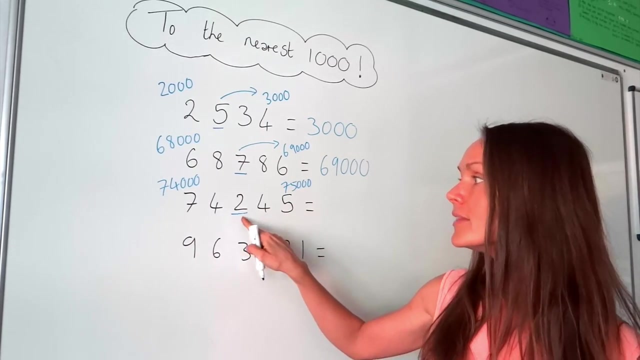 multiples of 1000, starting with the smaller one here. So the bigger one is 75,000.. So you might be able to spot straight away which one this number is closest to. but if you can't check that third digit there- the third one from the end, and this time it's smaller than five, which means we